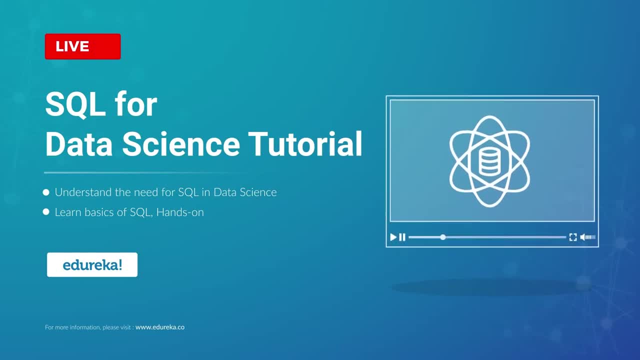 big players And all the companies used to have a license of SAS programming And it was a very powerful tool for data analytics. But the license of SAS was very costly. In 2009, I still remember it costed around three lakh rupees per desktop. 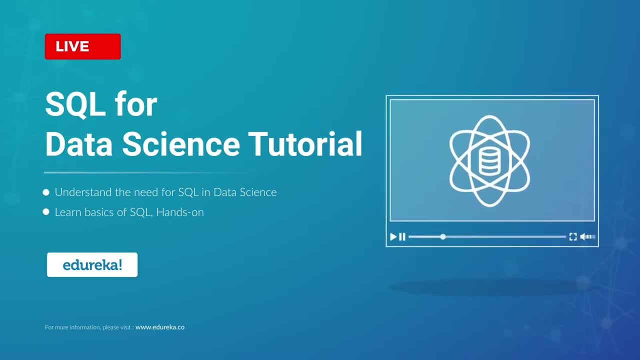 And for the enterprise. you can think of millions of dollars they just need to give to procure the software. But Python changed this whole history and R also changed this whole history. I'll talk about that as well, along with SQL, and why Python and R. I'm talking because of the word data science. 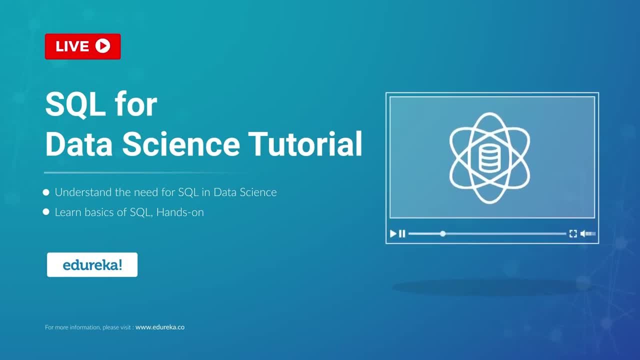 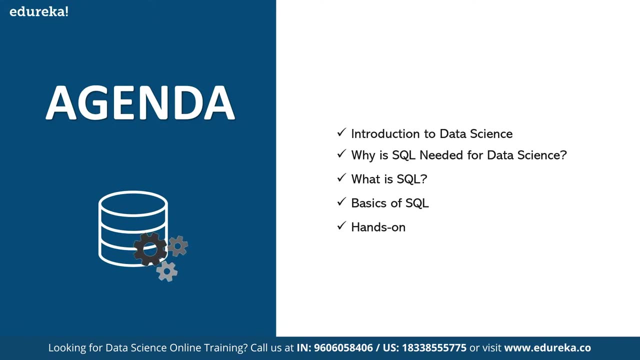 So let's move on with the slide. I'll go with the slides first and then I'll share my experiences of different areas. So we're going to work on what is data science, why SQL is needed for data science, what is SQL, some basics of SQL and. 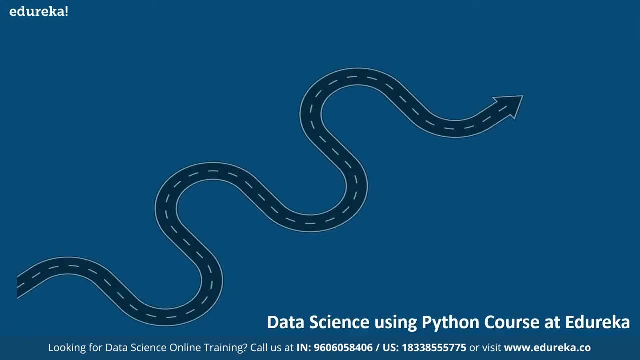 and I'll show you some commands of SQL that we need to write. I'll tell you the roadmap which is going to be covered. So first is we are going to learn what is Python. introduction to Python in corporates. some basic data structures in Python, like list, tuple, dictionary sets. some basic data structures. 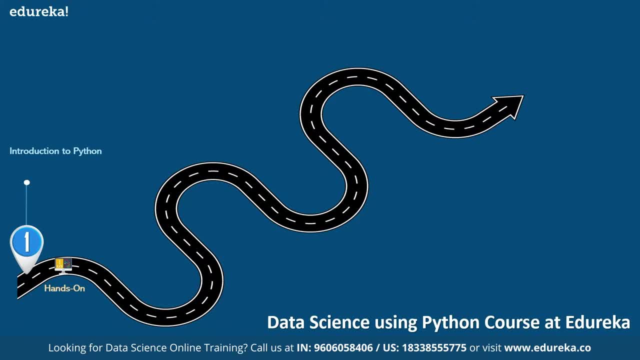 like data types in Python. what are the basic indentation rule in Python coding? What are the different types of variables we can create? how to write on the conditional logic using if loop while loop for loop. then we are going to work on. 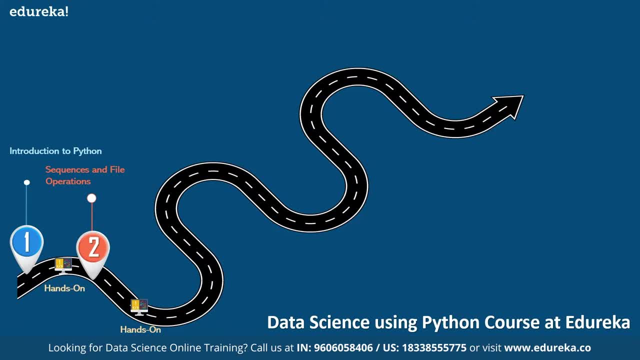 sequences and file operations. Sequences means any containers like list, tuples and dictionaries. They are the containers which can contain the huge amount of data. Like you can understand with the term arrays- In other programming languages they are called arrays- where you can store some data into it. Similarly, we have list tuples and dictionaries in Python. 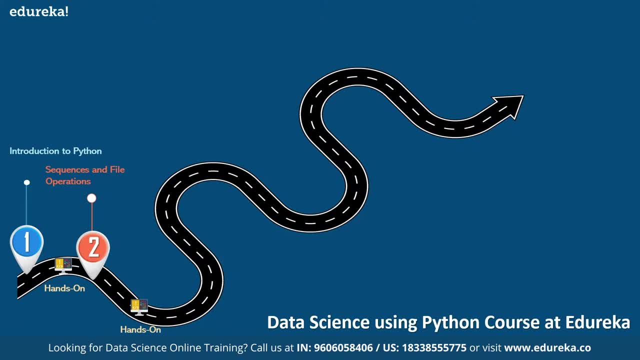 where you can store some data, And we are going to work on file operations, like basic file handling, opening a file, reading a file, filtering the contents from the files and the file operations. Then we are going to take a deep dive in functions. Functions are nothing but a reusable code. 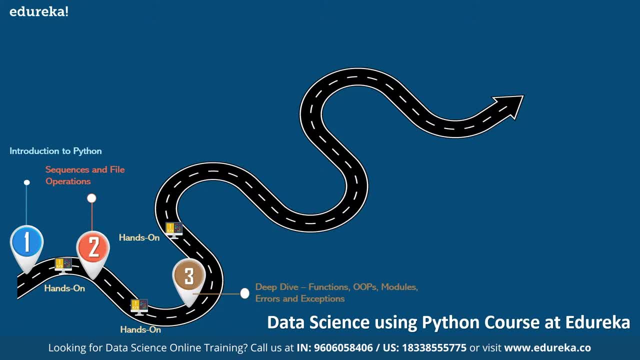 We are going to talk about different types of functions: arbitrary functions, lambda functions, object-oriented programming, concepts like abstraction, inheritance, polymorphism, exceptions and error handling. how to trap the error: There's a block in Python called try except else, and finally. So we're going to discuss on how to trap the exceptions. 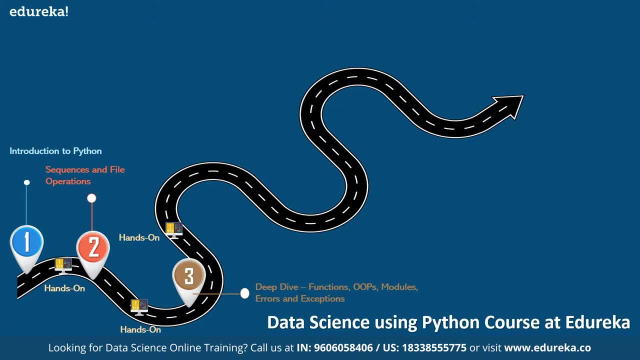 so that the end user will feel that okay, so is robust. then we are going to work on numpy, pandas and matplotlib. these are the three very important libraries in python which actually made python very popular. numpy is a library for numerical analysis. suppose you want to do any kind of a statistical and 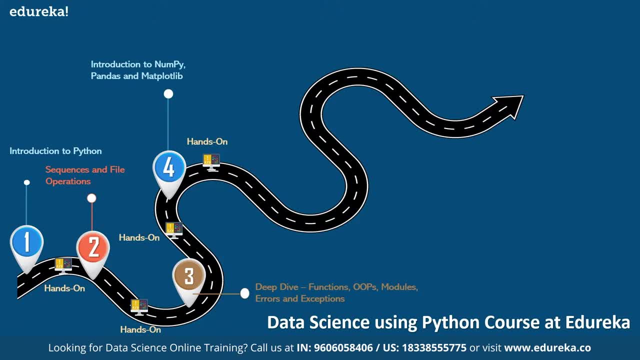 mathematical operation. suppose you want to find the p value, z score, iqr for outlier detection. you want to find out kurtosis, you want to find out standard deviation, covariance, variance, correlation map, confusion matrix. so all these things can be done through numpy. panda is a library for data analytics. suppose you have a data in an excel sheet or you have a data in a csv file. 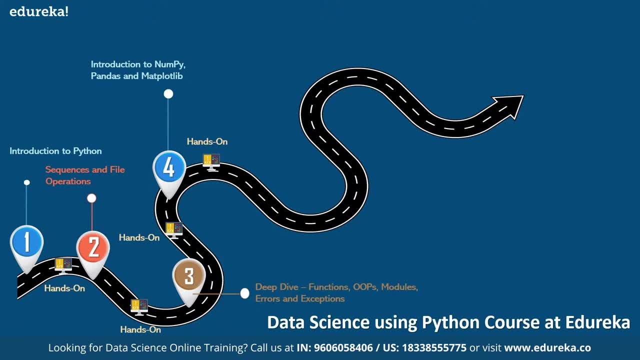 or you have a data in a sql database. you can fetch the data from that repository and get it into panda's data frame, and panda's data frame has got more than 500 plus functions to wrangle the data. wrangling means munging, joining, concatenating, filtering, subsetting any kind of operations on. 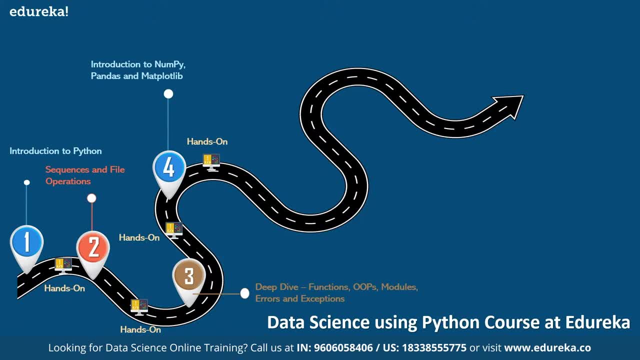 the data. matplotlib is a library for data visualization. suppose you want to plot a bar chart, histogram, line plot, scatter, plot different types of graphs. if you want to plot, you can write down the very simple lines of code. in few lines of code you can get the graph. that is done through. 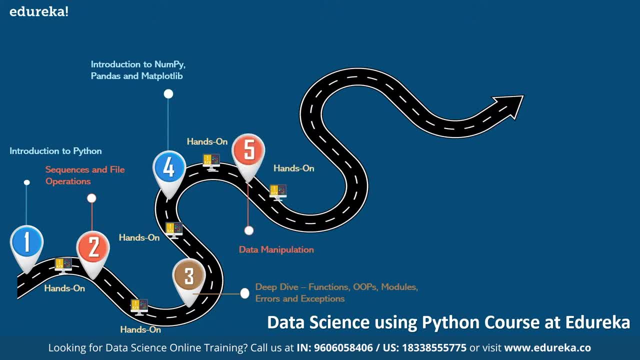 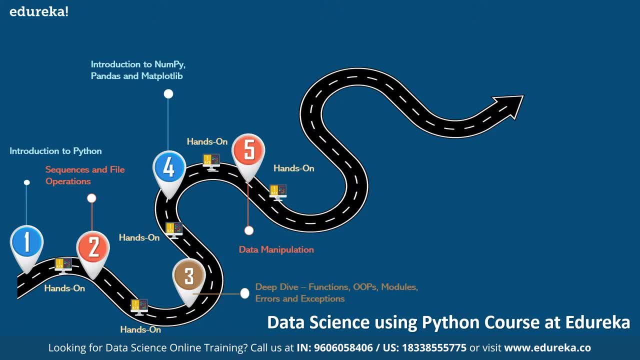 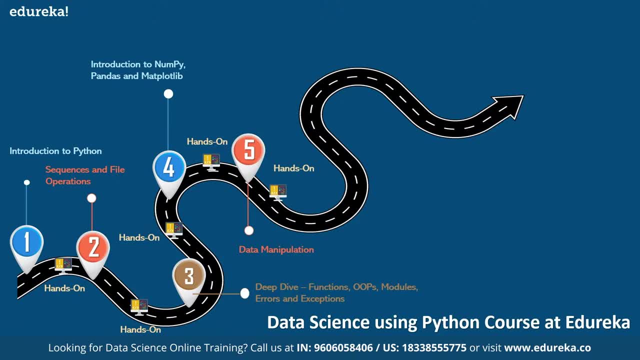 into it. you can use, through combination of these libraries, pandas, numpad, matplotlib. so when we use all these three libraries, we can wrangle the data and visualize the data in a easier manner. then comes machine learning with python. what is machine learning? you might have seen in youtube and 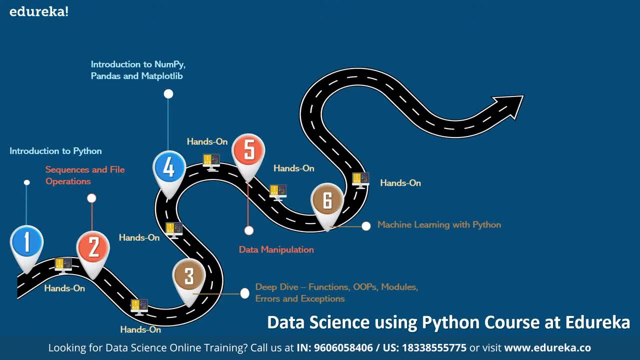 linkedin and on the other social media websites. artificial intelligence: machine learning- post graduate program in data science. so what is machine learning? let me explain you what is machine learning in a very layman terms. suppose you want to explain what is machine learning to a sixth standard boy who do not know much about computers? 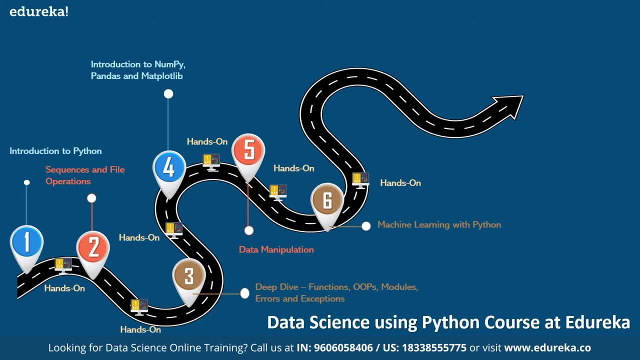 in simple terms, machine learning is predictive analytics. when we want to predict future based on historical data, we want to do machine learning or we are doing machine learning when you are predicting future based on historical data. suppose i give you last 20 years data of humidity, rainfall, temperature and crop yield, and if i ask you, what is a crop field in march 2023? 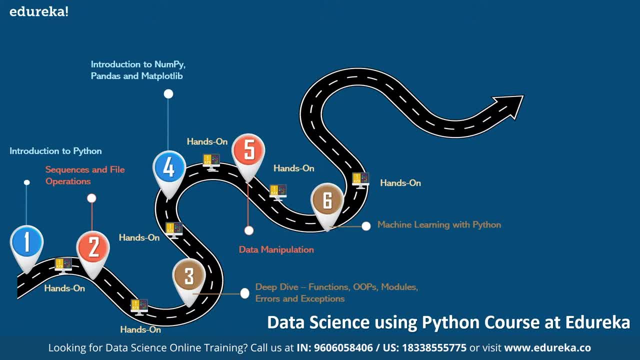 what you will do. you will use this historical data, find out the relationship between independent and dependent variables using statistical formulas and you create some kind of equation and say that crop yield is equal to 1.2 times of rainfall plus 2.3 times of temperature. 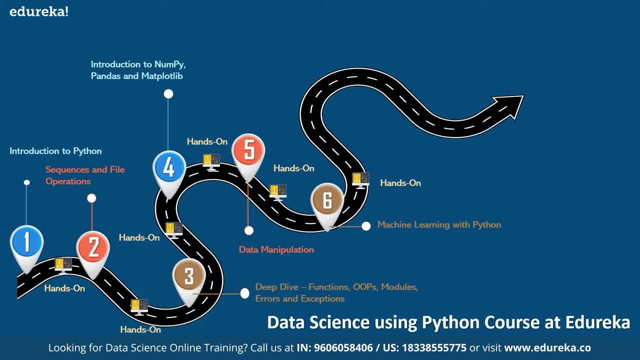 minus 1.6 times of humidity, plus some constant, you create some equation to map these independent, independent variables and use this equation in future to predict something, and that is called as machine learning. we are not in the era where machines have got intelligence, so all these movies i, robot or terminator- are just a science fiction. we are not in the era. 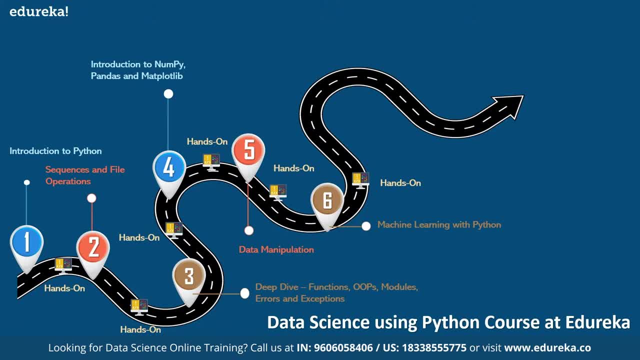 where machines can think and take decisions. we as a programmers are using some statistical algorithms like linear regression, logistic regression, decision trees, random forest, native classifier- there are so many of them. we use these algorithms to find the hidden insights in the data and mathematically equate some equation and use this equation for predicting things. 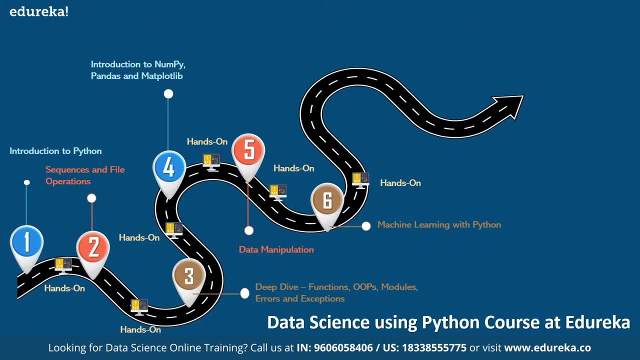 so the end user feels like that machine has got intelligence, but we as a programmers are writing down the piece of code, using these algorithms and finding the insights in the data and predicting future. and what are the applications of this machine learning? applications are uber cab or ola cab. when you book a cab, you come to know cab is going to reach you in 10 minutes. we are predicting. 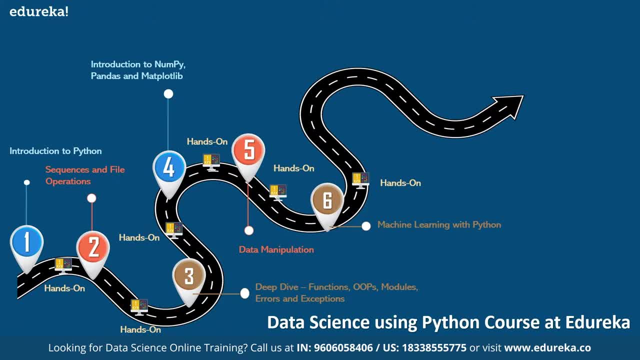 the system is predicting that the cab is going to reach you in 10 minutes, depending on weather conditions, depending on road traffic and all those things. go to amazon and buy laptop. amazon recommends you. why don't you buy a laptop bag as well? so this is what machine is predicting that. 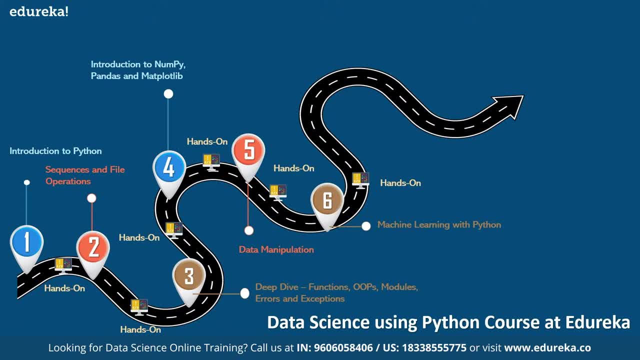 what next item you can buy and it is promoting their sales. there is no human intervention and machine learning is a subset of artificial intelligence. artificial intelligence is anything which is mimicking human behavior. so anything you are trying to convince foundations, this is the mac mimicking human behavior. so anything you are trying to mimic like a human, it is coming under. 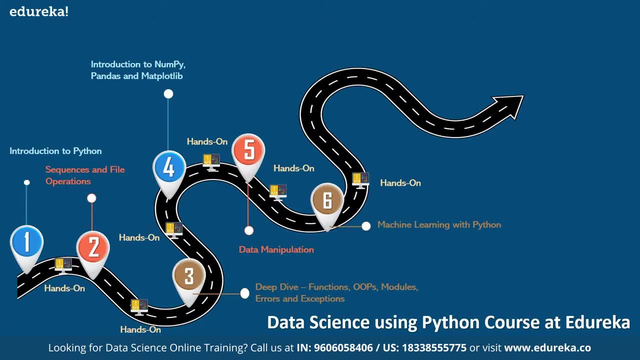 the umbrella of artificial intelligence, and machine learning is a subset of artificial intelligence. subset means it's a part of artificial intelligence. deep learning is a subset of machine learning. there's another term called deep learning. deep learning is a subset of machine learning where we are talking about images when the data is multi-dimensional, like three-dimensional. 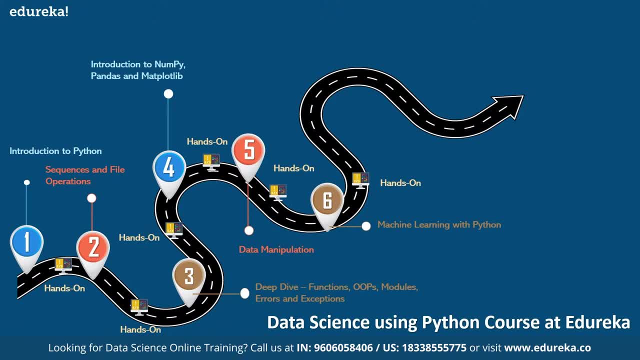 like rgb values in a pixel. so when we have a three-dimensional data, machine learning algorithm fails, then we have to rely on deep learning. there are different libraries for deep learning, like keras, tensorflow in python, and deep learning is primarily focusing on computer vision or handwritten text identification. text conversion: german to english text translation image. 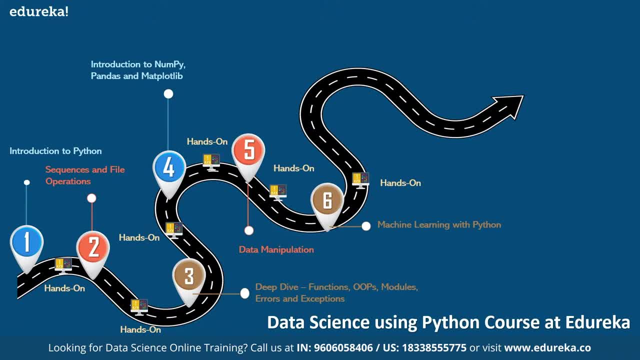 colorization- coloring a parrot from a gray style to a colored image. so all these things comes under the umbrella of deep learning. so machine learning is a subset of artificial intelligence. deep learning is a subset of machine learning, and machine learning primarily deals with predictive analytics, association rules and recommendation engines. 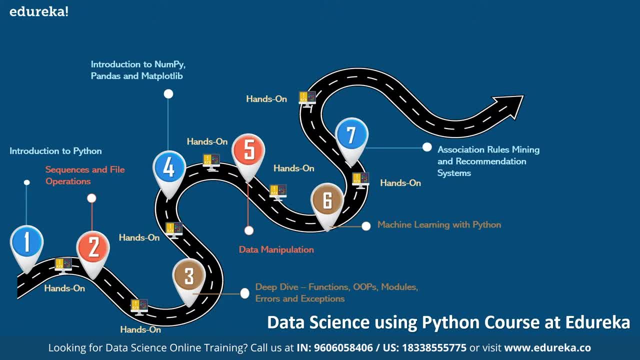 as i was talking about, it's also a part of machine learning recommendation engines. we are using an algorithm called a priory a-p-r-o-r-i, which is used by amazon to recommend the products to the end customer. so this is again a component of good points. key supports: timetable argument is where we don't use conventional. 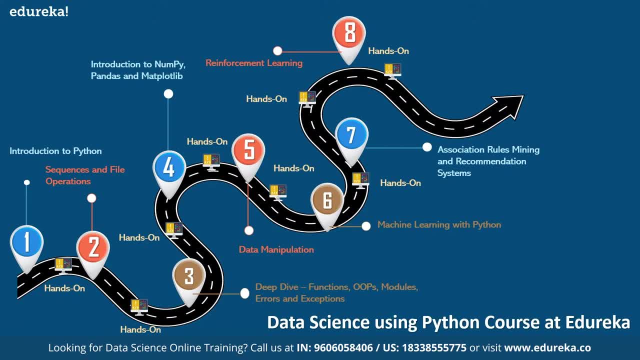 progressive computer computing heatποιens running the différence with a認 spirituality proposition, non-primitive compartir, which also allows some logistic initialization s sebeliyo attention, person quantification, difficulty, flexibility, ρη understanding different clusters. so all the clustering algorithms like k means clustering, c means clustering. 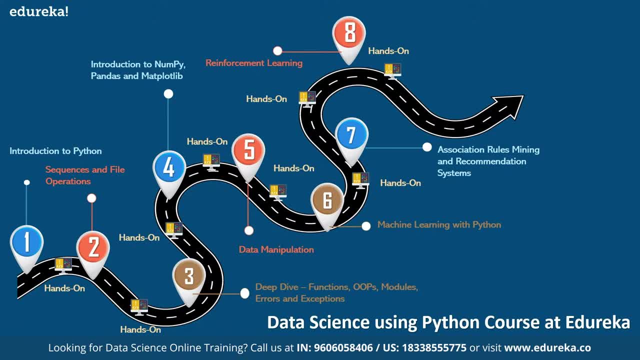 agglomerative clustering comes under unsupervised reinforcement. learning is learning with experience, slow and gradual learning. for example, manless car: the scientists used to give some hundred images to the car on the daily basis and car take some decision. these decisions may be right or may be. 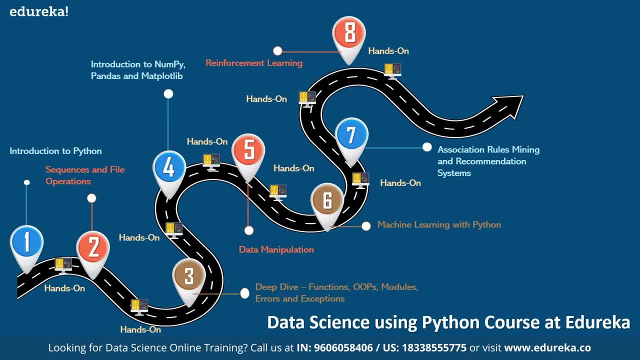 wrong and keep on giving hundred, hundred images on the daily basis. and for the wrong decisions we give some penalty and some policy that next time this should not happen and keep on supplying images. and time has come where machine knows millions of images. what action to take so that 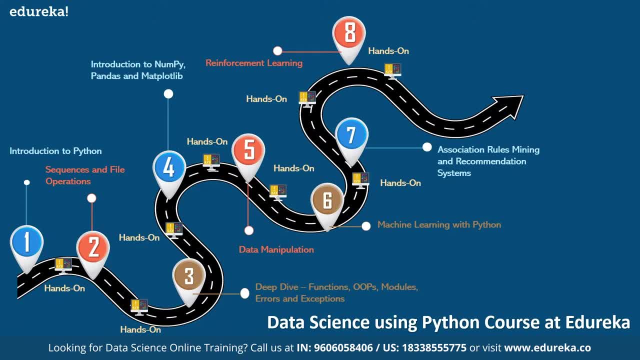 is called the reinforcement learning. it's an area of research. all the innovation-based companies who are into innovation. they use reinforcement learning, like chatbots. you might have seen the chatbots become smarter and smarter- gaming companies, where games become smarter and smarter day by day. so that is called as a reinforcement learning. 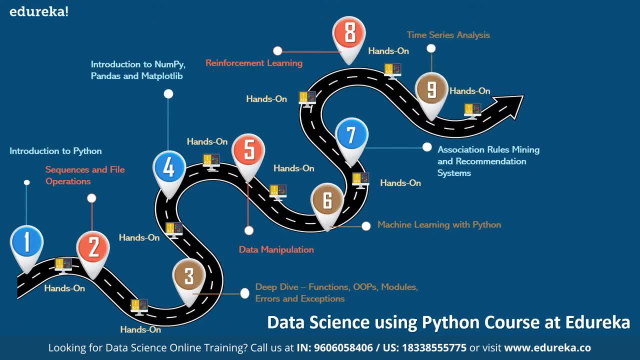 you then comes the time series analysis, so we have stock data, like if you want to predict the stock price, what is going to the stock price tomorrow based on the historical stock prices- then we are using a time series analysis and then model selection and boosting. so when we do all this, 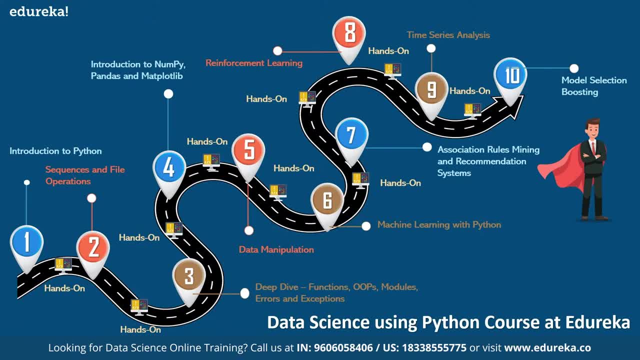 machine learning task and we found the accuracy is not coming good. we try to improve the accuracy by using xg boost and add a boost algorithms. so in order to get a better accuracy, we use different algorithms to improve the accuracy of the data so we have stock data, like if you want to predict. the stock price, then don't wait for this model. we have to create this Indo now. let's have stock anytime, so maybe 10 to 20 on the way to understand how the cost price100 plus this data doesn't necessarily mean the cost price comes from the stock price. now. I'm just saying you should go, look at the results And when you sort your head and let's say a stock price sample, we have goodicios. I think our concern right now is what is a complete data science and the market? sure, sandy at the candle is something which has built in the goal month to improve that. 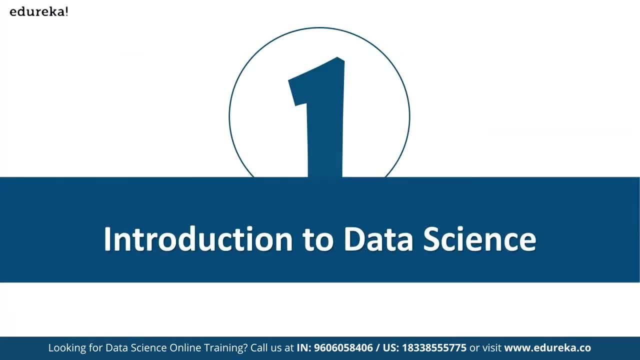 well, see that is called boosting algorithms and then we have a final project. what is data science? data science is a process that I've been: useful insights with a good time auto saw real problems. so imagine I've given you that came Si details of a customer who are there with Amazon like a gender location. 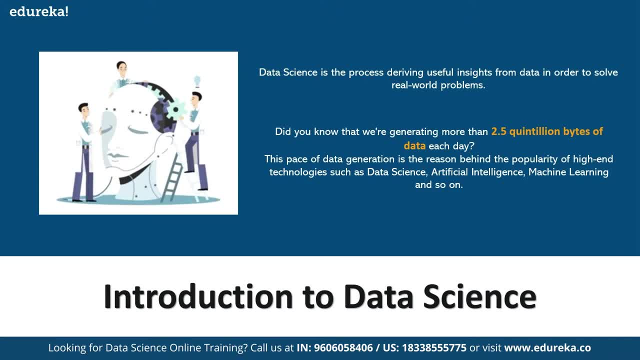 address, last purchase histories, and I've given you millions of customers that are you So imagine. I have given you the KYC details of a customer who are there with Amazon, like age, gender, location, address, last purchase histories, and I've given you millions of. 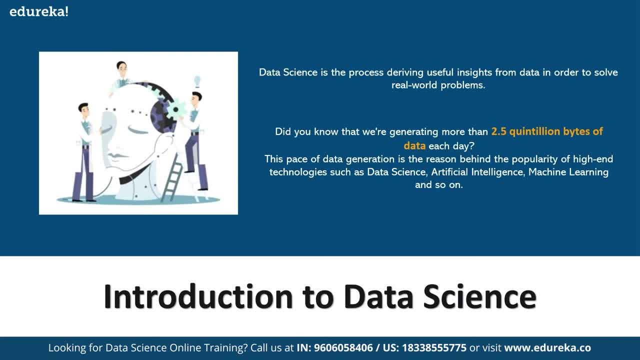 customers data to you and you want to get some insights into it and you want to figure it out. Laptop is bought by what age group? what is the age group of the people who are primarily focusing towards purchase of laptop, or in which season what products were sold most? 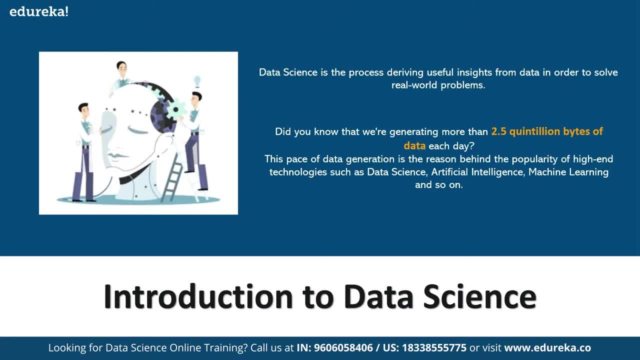 so all the real-time problems can be solved through data by finding the hidden insights, and data science is just a process of finding that hidden insights. Do you know that we are generating more than 2.5 quintillion bytes of data each day? So that's a huge amount of data we are generating on a daily basis worldwide? 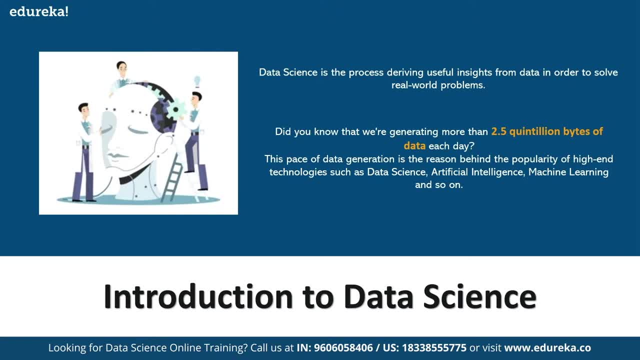 This space of data generation is the reason behind the popularity of high-end technologies like data science, artificial intelligence, machine learning and so on. So it is impossible for a human to find the hidden traces in this much amount of data. That is the reason we are using a lot of softwares and tools and techniques like DevOps, like 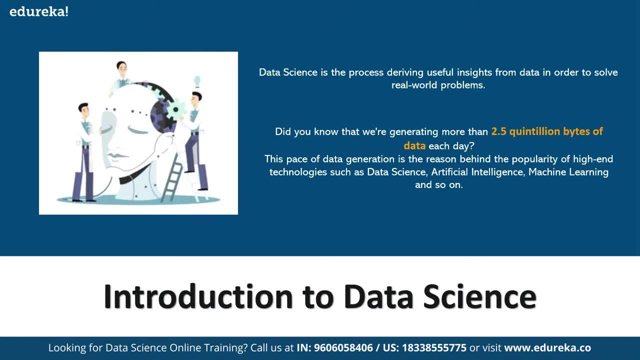 we are using Kubernetes, we are using big data like Hadoop and Spark environment to process this amount of data And we want some programming languages to find the predictions on this data, And that is the reason Python and R became popular. So data science is a holistic view where it incorporates data acquisition. 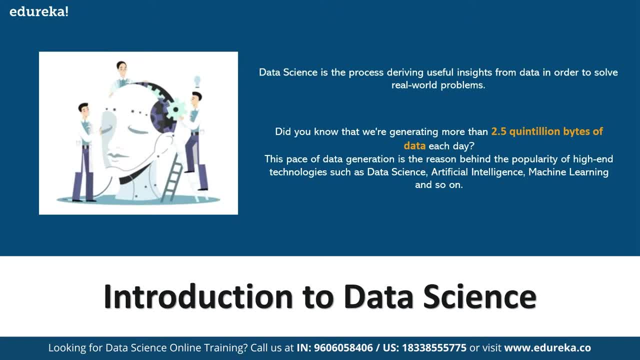 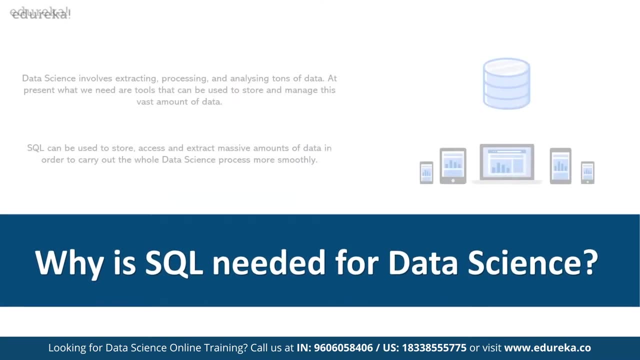 Data gathering, data mining, then filtering, then doing some hidden insights, data visualization, getting some predictions. So data science is a broader term which encapsulates everything. Now why SQL is needed for data science. Data science involves extracting, processing, analyzing tons of data. 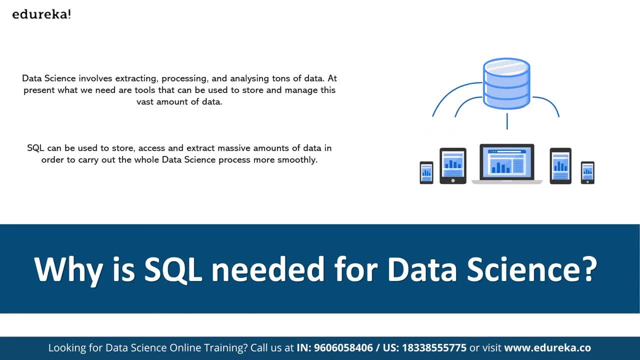 At present, what we need are the tools that can be used to store and manage this vast amount of data. So SQL is nothing but our relational database. So SQL is nothing but our relational database. Like Oracle, like MySQL, it's a relational database having data stored in a form of an. 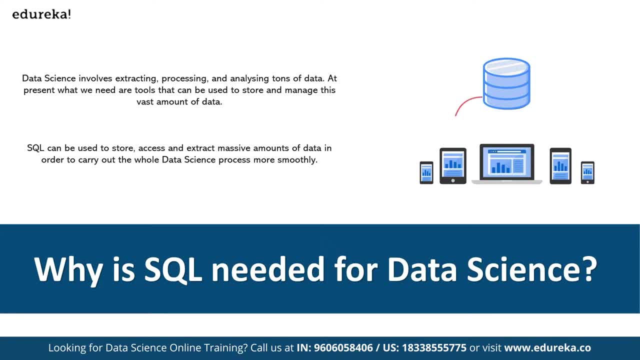 Excel sheet like an Excel sheet in a form of tables, where rows are called tuples, column headings are called attributes And we store the data in a form of a tabular format And then we can use the column headings to filter the data, or we can use some different. 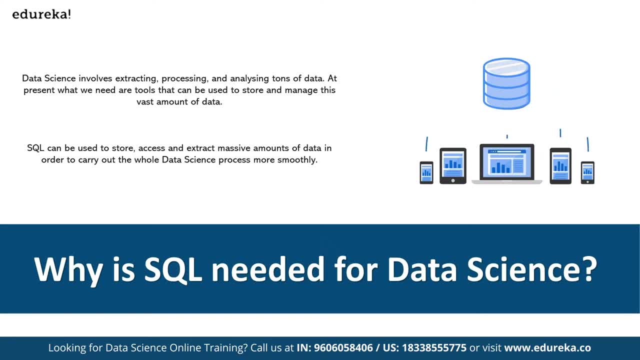 commands in SQL to process this data. Data ranking commands are there in SQL and data manipulation commands are there. So data science involves data collection. Structuralize involves extraction of the data, processing of the data and analyzing it, And for that SQL is used. 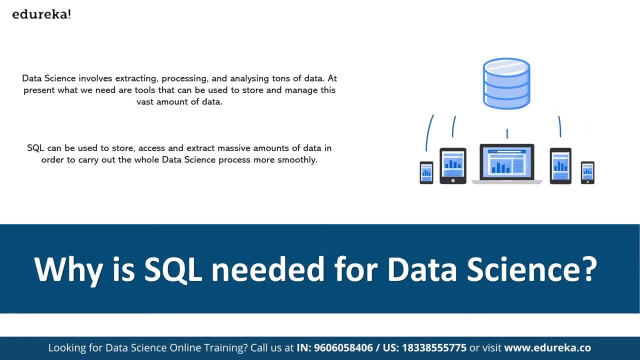 SQL can be used to store, access, extract massive amounts of data in order to carry out whole data science process smoothly. So, as I told you, we need to fetch the data from a repository first, Then we need to process it, Then we want to find some hidden insights into it. 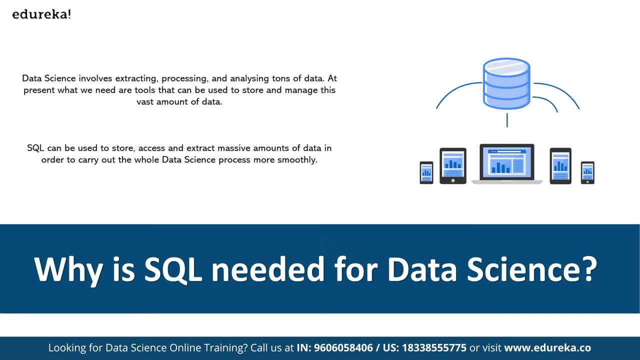 Then we want to predict it, And for all this we need a good tool where we can store the data and do some data wrangling queries, And for that we use SQL. Of course, for prediction we use programming languages like Python. 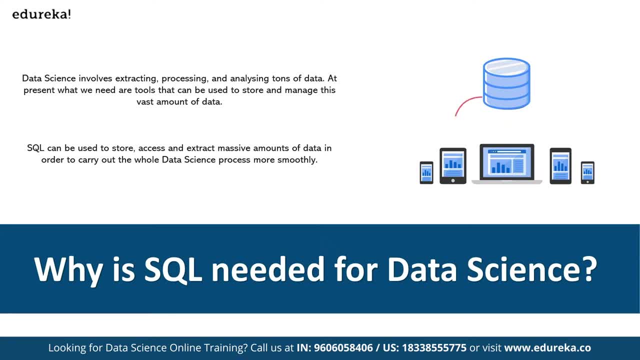 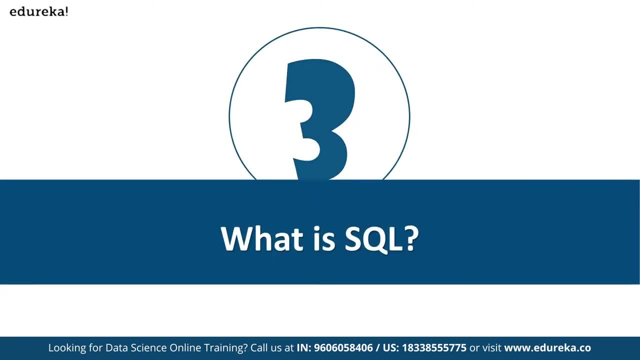 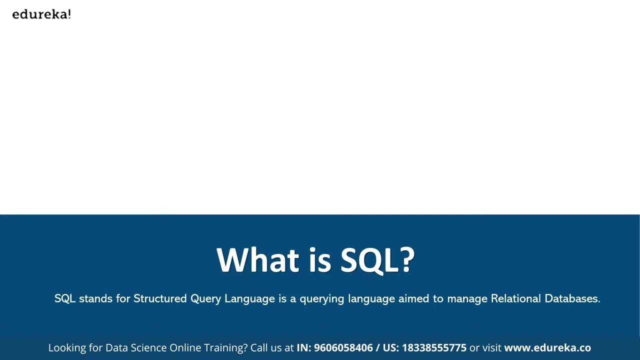 But we need some data to predict Raw data, on the top of which we are predicting that raw data is supplied by SQL. What is SQL? SQL is structured query language. It's a querying language aimed to match relational databases. So relational databases means you can perform some joins like inner join, outer join, left join, right join. 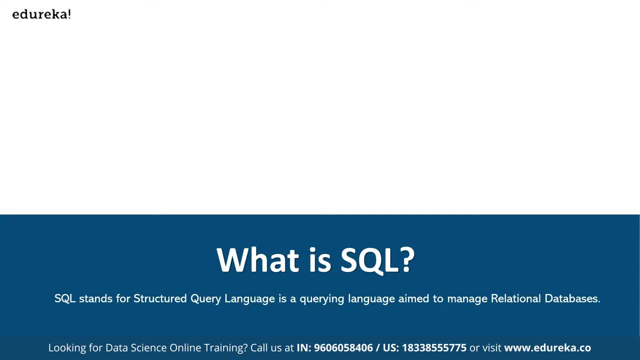 based on some primary key, foreign key, Secondary keys. So there are a lot of terminologies in SQL again, like first normal form, second normal form, Boyce-Cord normal form. We have a lot of commands in SQL. I'll show you the cheat sheets in SQL that we can use to write on different commands. 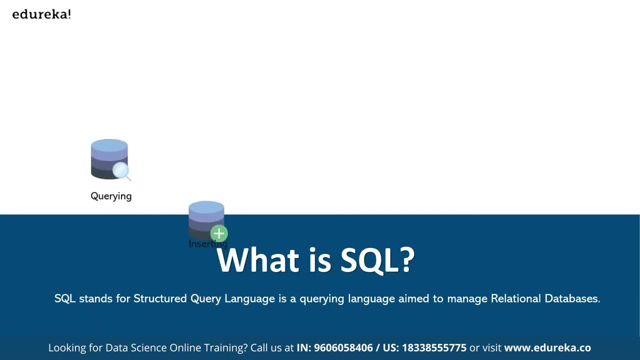 Okay, So what is SQL? SQL is all about query, Inserting the data into the tables, updating those tables, deleting the data from those tables, extracting the data from those tables. So RDBMS is a data Management tool where data is stored into different tables. 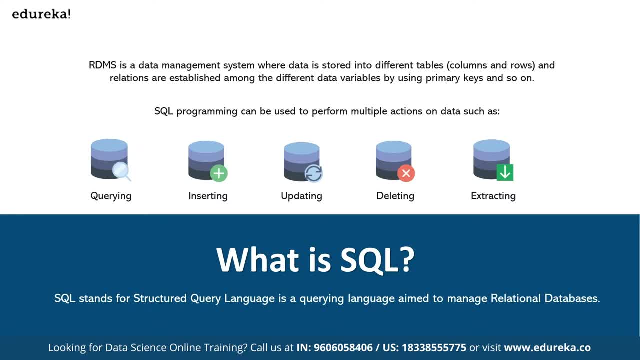 So we have columns and rows, We have different structures in which we can store the data and relations are established among those data variables using primary keys. So in one table it is called as a primary key and other table it is called as a foreign key. 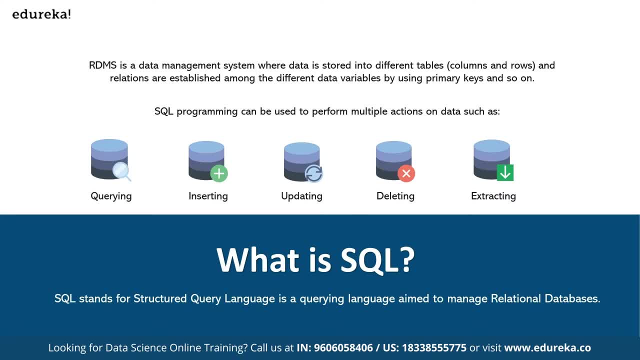 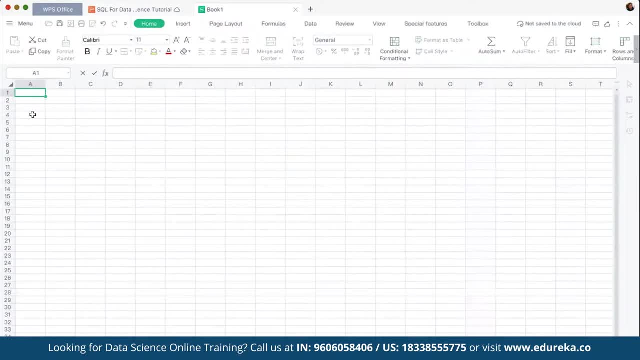 For example, you have one data which is in a form of employee data. So let's say I create one data set. Let's say I have one table, table one or employee table Having column headings as employee ID and age and salary. 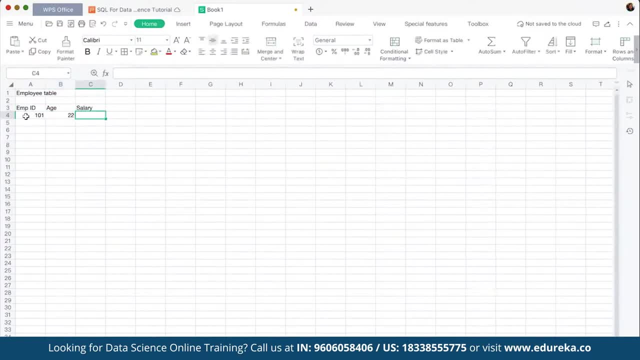 Let's say I have an employee ID 101,, age is 22,, salary is 20,000.. 102,, age is 23,, salary is 23,000. and 103,, age is 41 and salary is 44,000.. 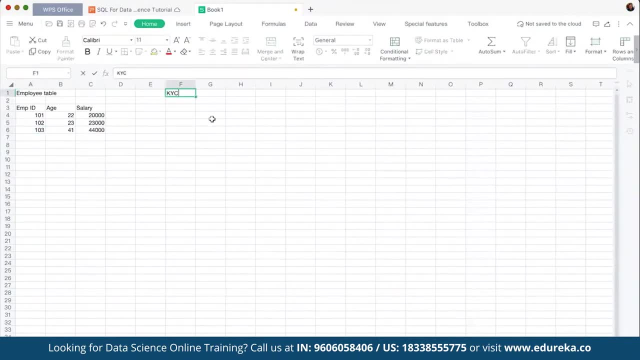 And I have another table called KYC table And in this we have employee ID, name and gender. 101: name is Amit, gender is male. 102 name is Sumit, gender is male. 104, Sunita and gender is female. 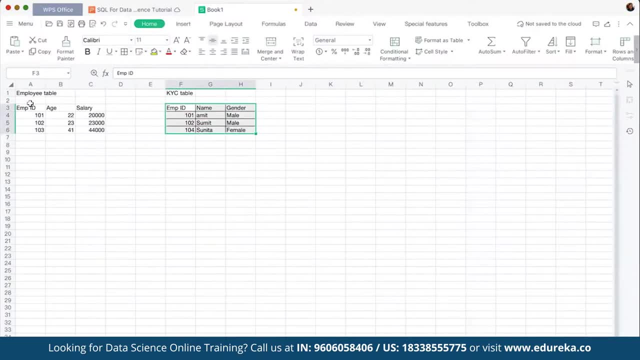 So let's say I have two tables- This is one table and this is another table- And I want to perform some inner join. So inner join will do what Inner join will give common records. So I'll join with employee ID, So I'll get an employee ID. 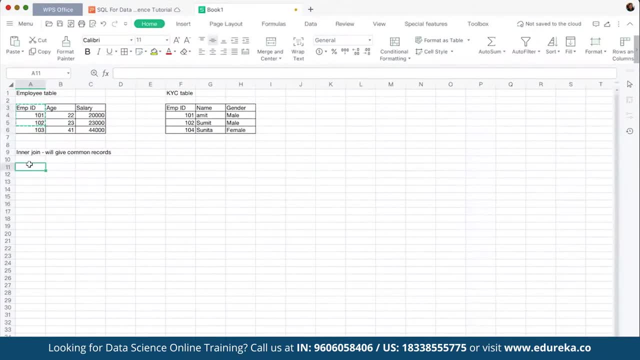 What is common in both of them? We have 101 and 102. And we have name and gender, age and salaries And we have name and gender. So this is going to be the output for inner join. We have common records from both the tables will be fetched and we get a holistic view. 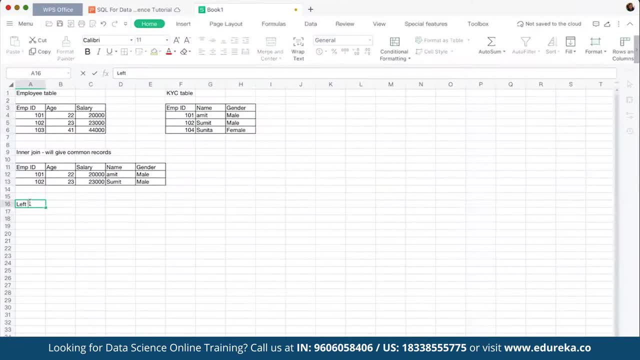 Then comes the left join, Left join will do what It will find. take complete first table and matching from set. So we'll get everything from here And we have matching here as Amit and Amit here, And this is going to be any. 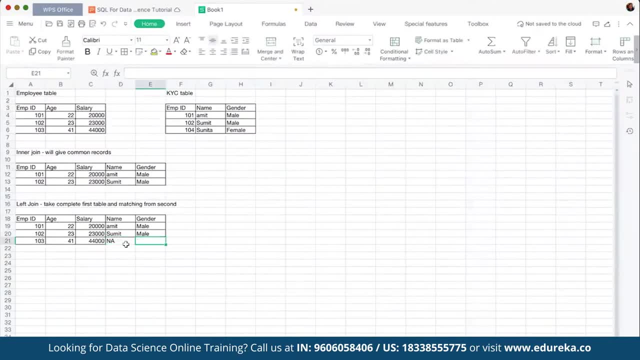 Any means missing value. In Python terminology it is called NAN or in R terminology it is called any. Any means missing value. Similarly, for the right join, We get all the data from the right and the matching from the left, And similarly we pull out our join. 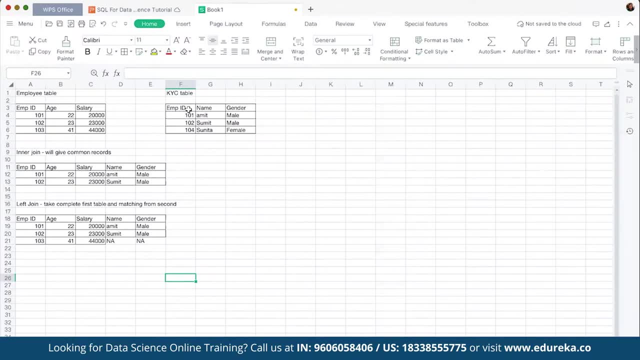 But these queries can be written like select star from table one, select these columns from table one and table two where age is equal to something. So we can use select queries to filter the things and we can write down the join queries to join the different tables. 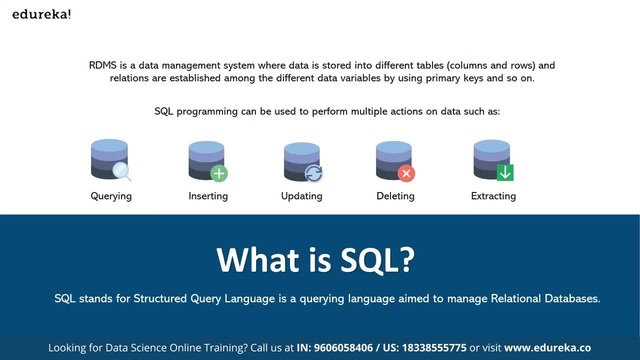 So these are primarily operations we perform on any SQL database, Like querying, Inserting, updating, deleting and extracting. SQL programming can be used to perform multiple actions on such data, So we can use PL SQL for writing down the procedures in SQL. 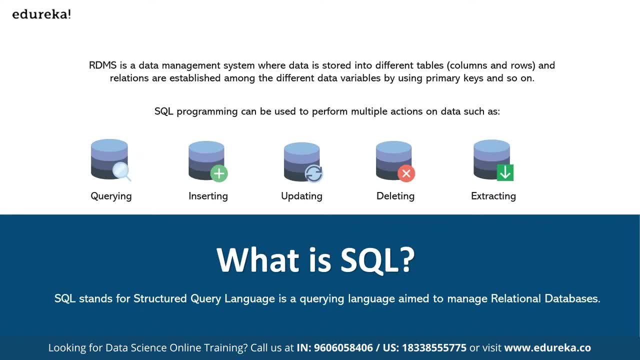 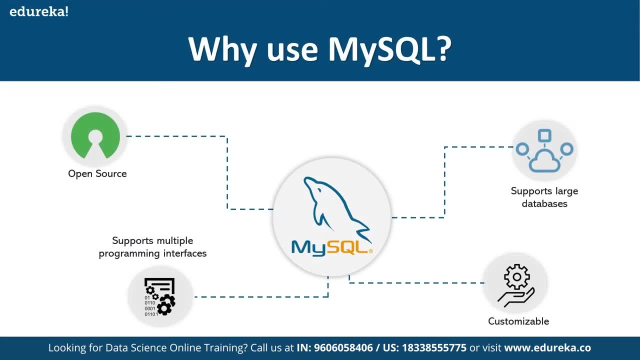 And SQL itself is a big ocean where you can do a lot of things in terms of database management. So why do you use MySQL? Because it's an open source. MySQL is a relational database. It is open source. It can support huge amount of data sets. 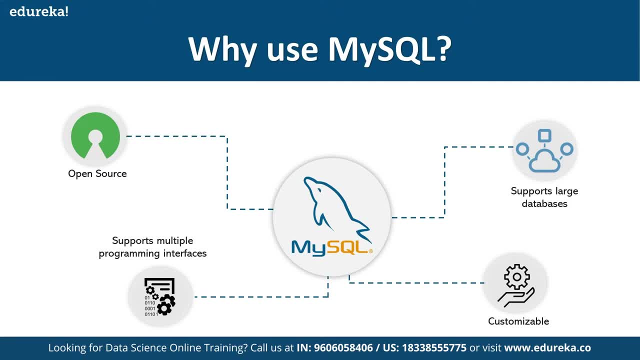 It can support multiple programming interfaces. You can connect MySQL with Python, You can connect with NET, You can connect with Java. So any programming language can connect with MySQL using connection string and fetch the data from a repository. And we can very well customize MySQL as per our needs. 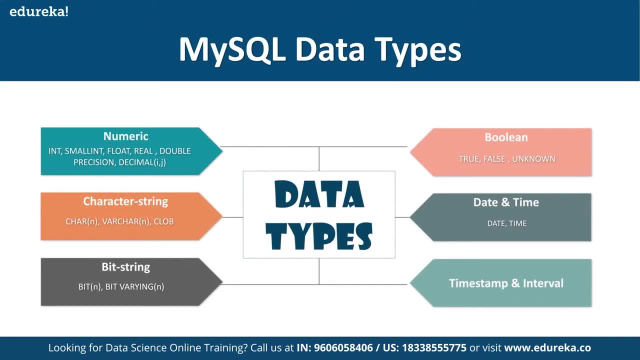 So there are different data types in SQL, Like numeric types, where we have integers, small int, float, real, double precision and decimal. We have corrector data types, We have varcars, We have blobs, We have 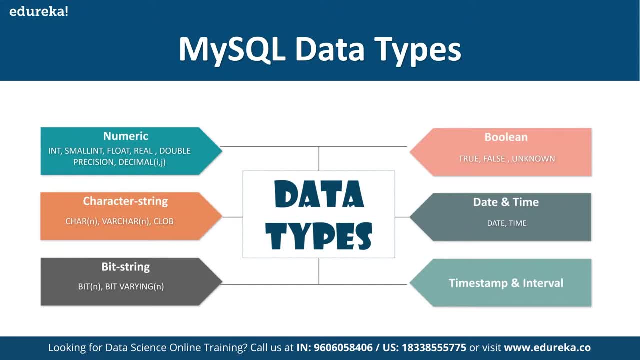 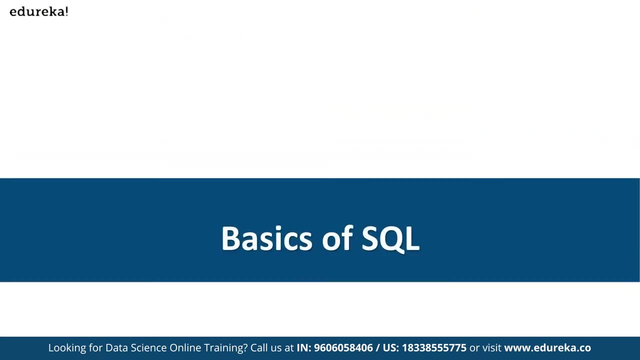 We can store the data which are bits bit varying. We can store Boolean data- true, false. We can store date and time formats. We can store timestamp and interval, So it can store any kind of data having different meanings. Now, if we talk about basics of SQL, we can use create database name from: 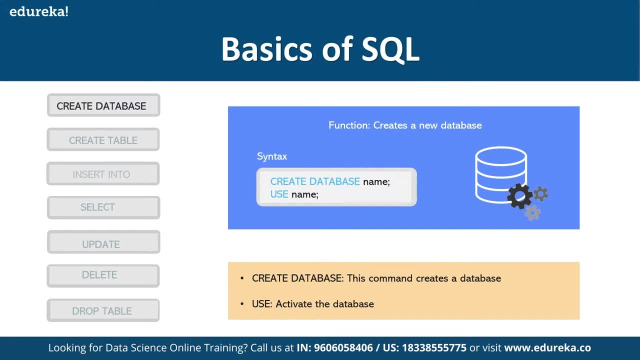 Create database name and we can use that name to use the database. So create database command is used to create, Activate the database and use this to activate the database. Similarly, we have commands to create a table, create table, table name and different variables in the table with very various columns in the table.